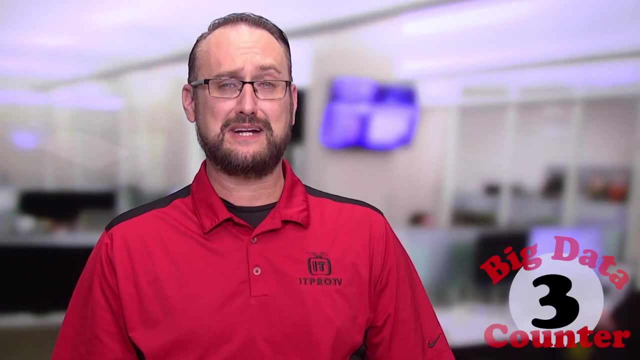 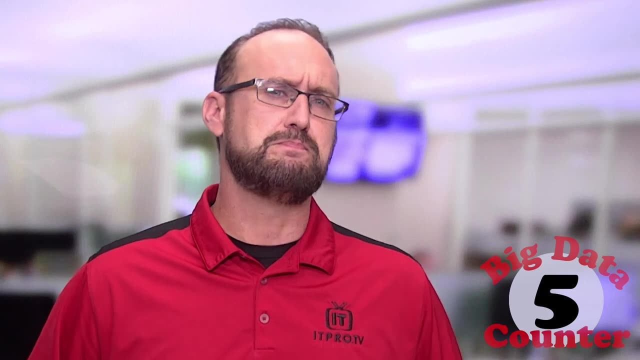 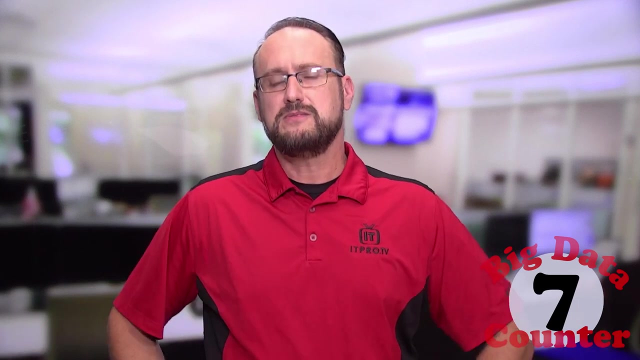 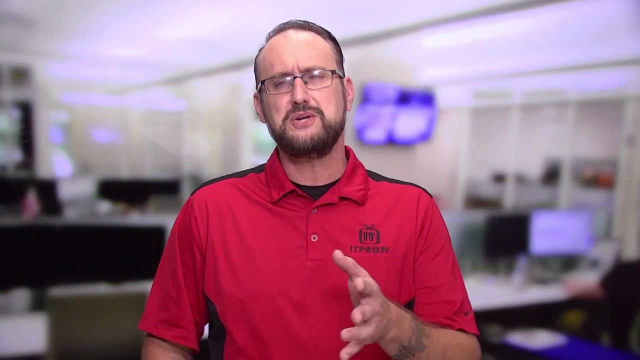 I kind of feel like I'm going to say big data a lot in this episode. I want to talk about big data-specific technologies and we'll take a look at some of the big data-specific roles that you'll see in the industry. So big data, What is it? Well, it's defined as extremely voluminous and complex data sets, And you will see more formal definitions, usually in three or more Vs. Some of the most commonly agreed-upon Vs are volume. 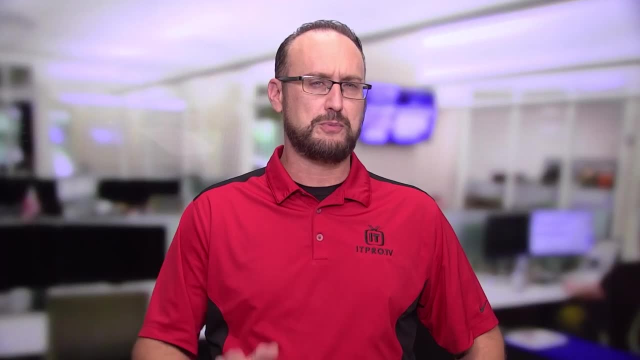 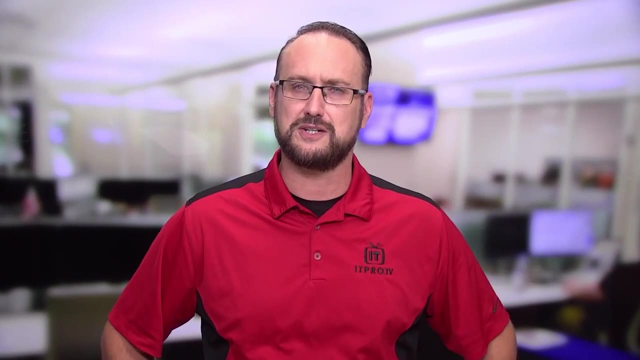 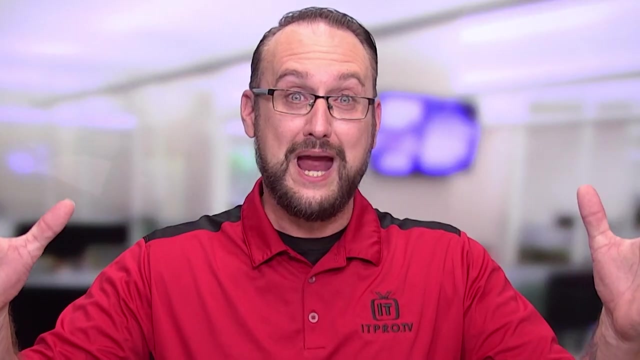 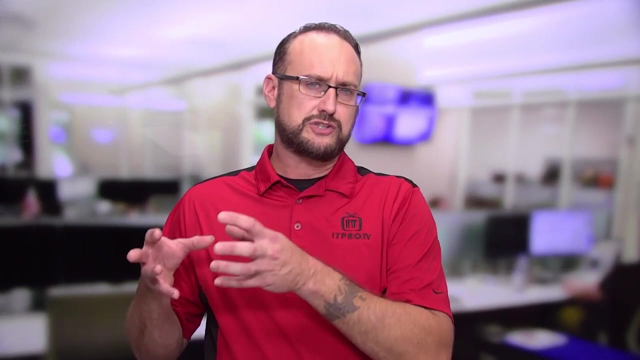 Volume means large amounts of data from multiple sources. Then there's variety- multiple types of data, typically structured, unstructured and semi-structured. And then there's velocity, And velocity is the speed at which the data is being generated. But wait, there's more. You may or may not see additional Vs like, for instance, veracity- the extent at which the data is correct or can be trusted. Then there's variability. 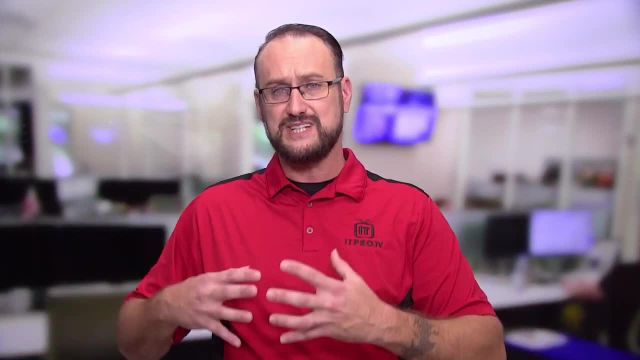 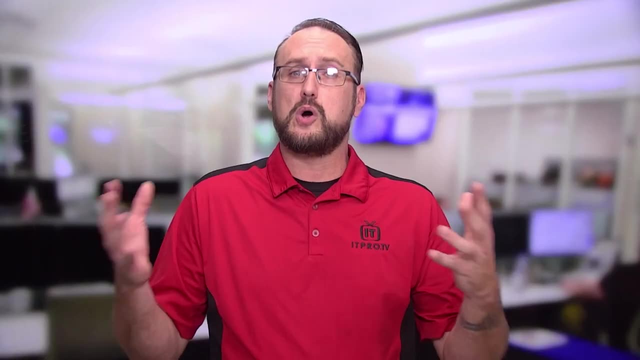 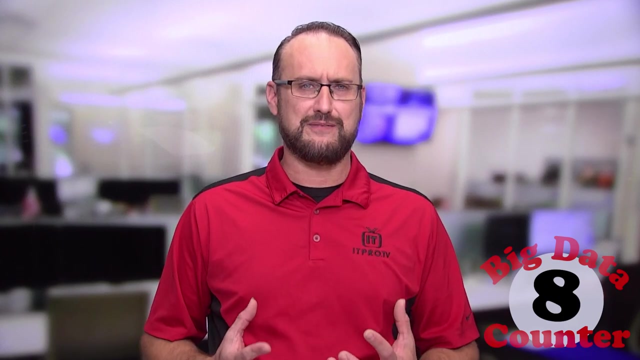 And the variability is the difference. There are different ways in which the data comes in and the inconsistencies. Sometimes data comes in fast, sometimes it comes in slow and sometimes it's all over the place. all different types of data. And then there's a very important part of big data: is making sense out of that data, through the V known as visualization. 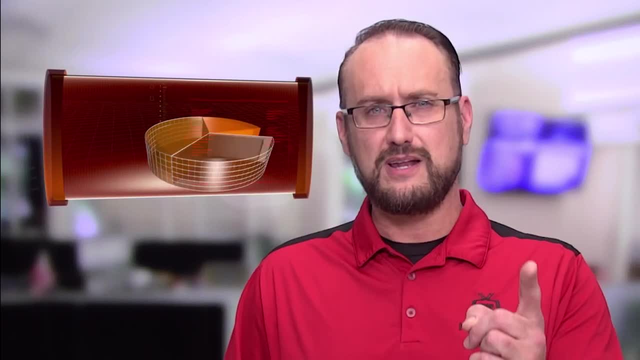 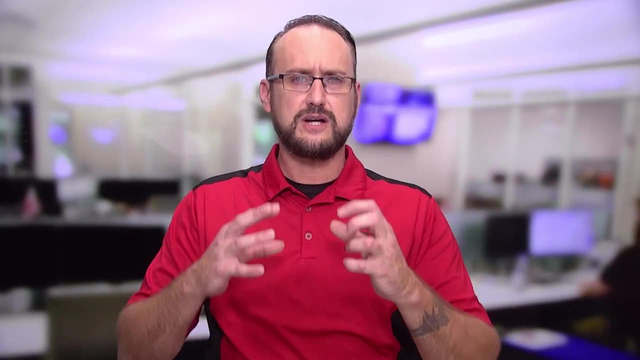 We've got to be able to consume the information to gain the last one, which is value, And that's the business worth of the data. What does the data mean to the company? Can the company actually use it? Can the company actually make sense and utilize this data? 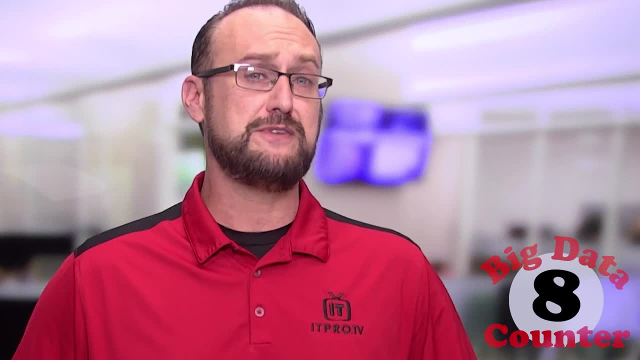 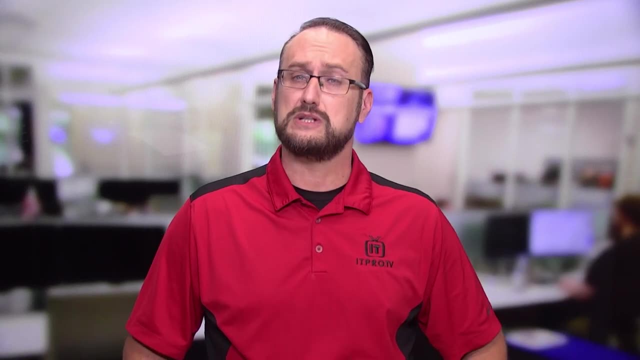 So what do all these Vs add up to? Well, let's talk a little bit about the benefits of big data. Here's some examples. For instance, through applied analytics, you can take a look at identifying patterns and relationships. Think about IoT. 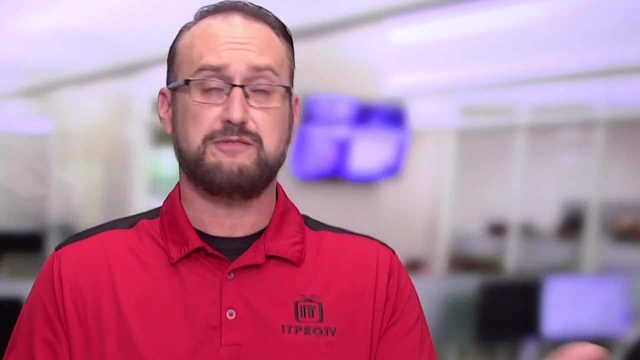 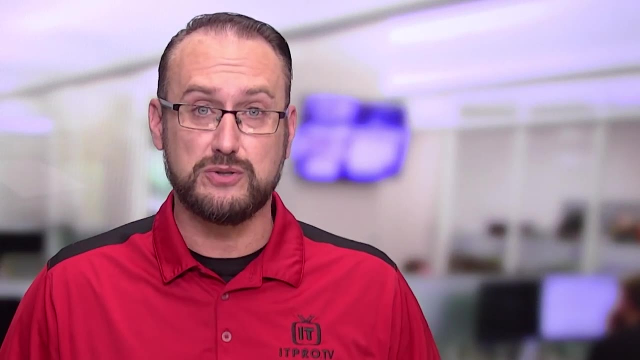 IoT is so important. today We have millions and millions. In fact, by the end of 2020, they're expecting 20 billion IoT devices, so we can generate things like IoT sensor data, you know, in mass quantities, Mass quantities. 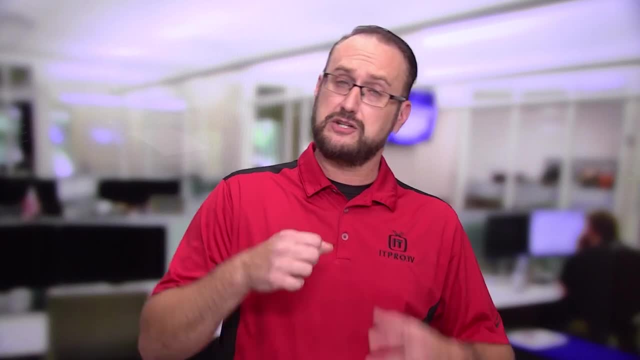 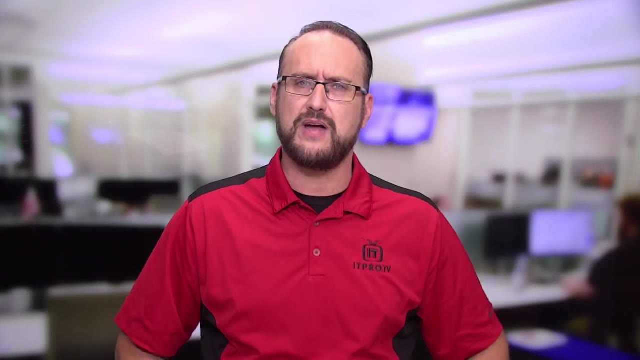 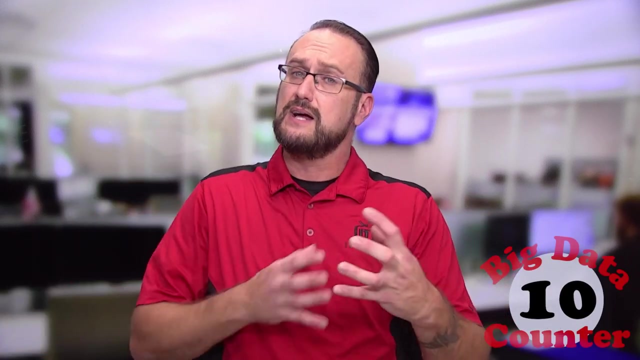 The other thing is customer analytics. Have you ever gone to Amazon and you purchase something and then you find out? the next time you visit Amazon, they put something in your suggestions and you're like, wow, I really like that. Well, Amazon has over 300 or more million customers and they scrape all of the information from big data, identify customer trends and use that to make suggestions, among many other things. 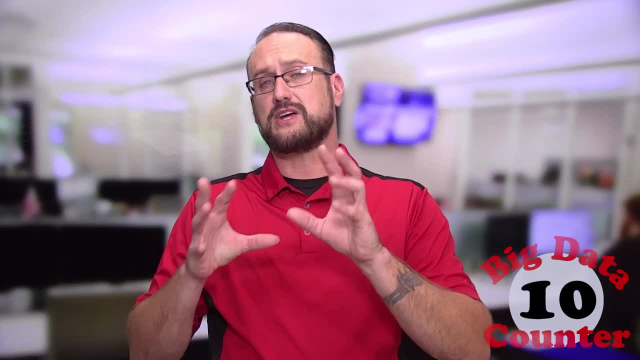 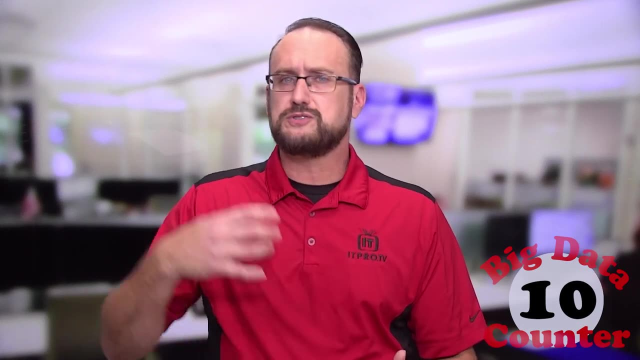 But then there's also operational analyst, analytics. Remember that the company, if they can identify this information, Yeah, Yeah, Yeah, They can identify trends, maybe improve workflows, maybe reduce costs. These are just some of the many benefits of big data. 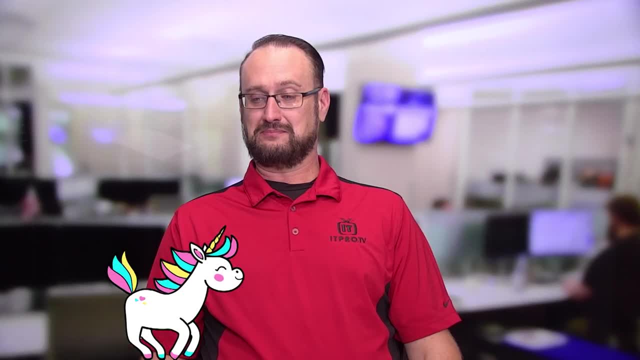 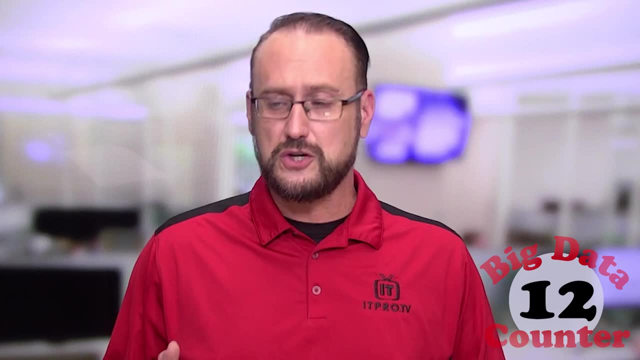 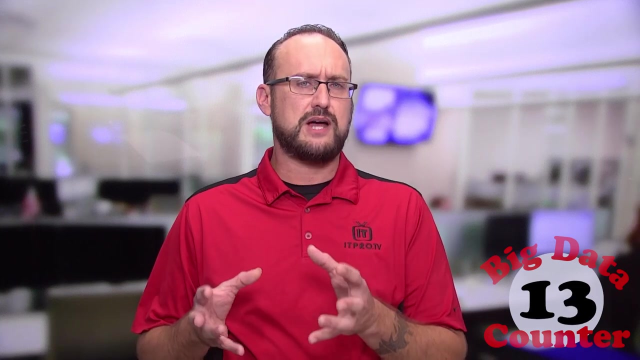 But it isn't all glitter and rainbows. Big data is still relatively new technology and there are challenges. Take, for instance, traditional software. For instance, when it comes to big data, traditional software does have its limitations. Some of the limitations: 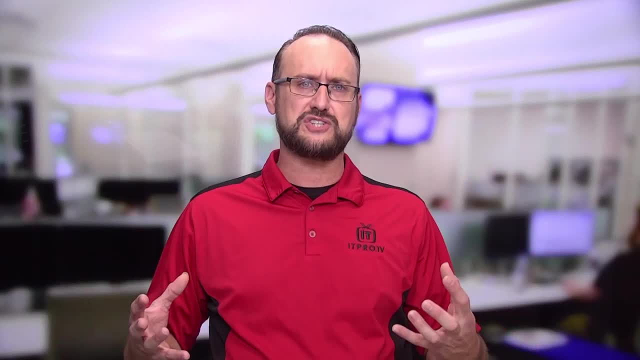 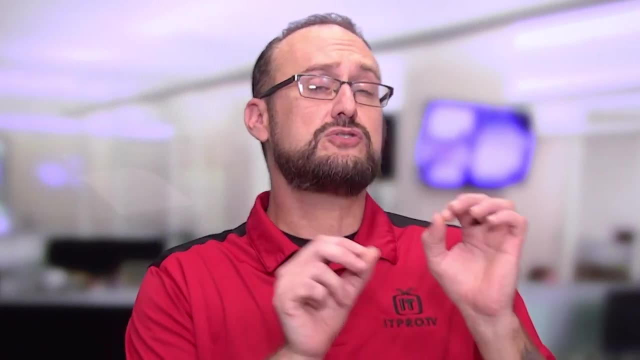 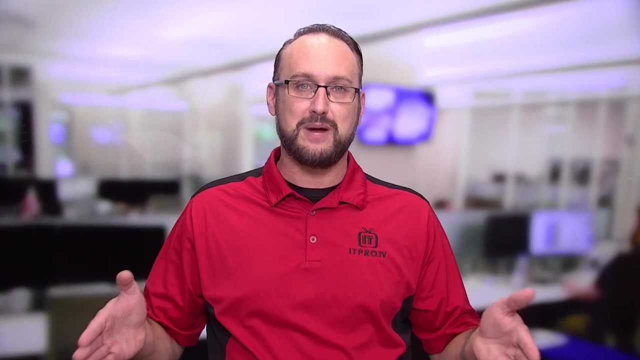 Are: how do we capture those large amounts of information? How do we store that information? And then, once it's stored, how do we maintain that information? Now the other thing is, traditional software isn't really constructed to process large amounts of information. 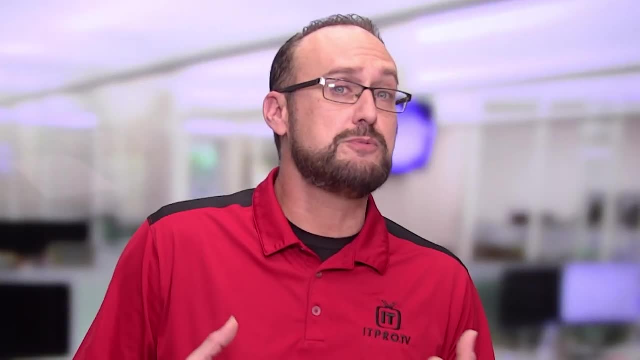 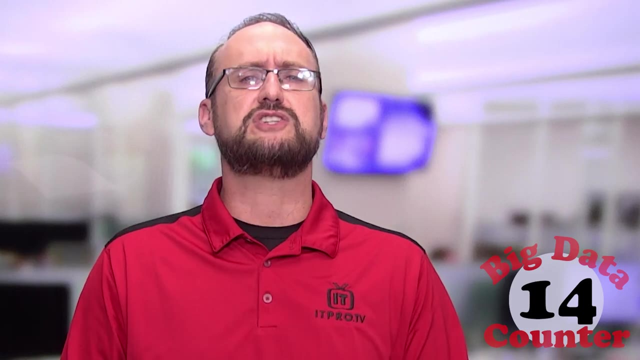 If you think about it, when you compute, when you use a computer, typically you process information in megabytes, maybe gigabytes, But with big data we're talking processing information in petabytes and beyond, Petabytes and beyond. Then we have to again make sense of that information. 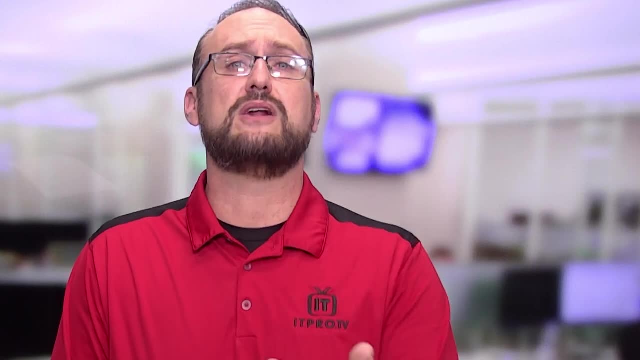 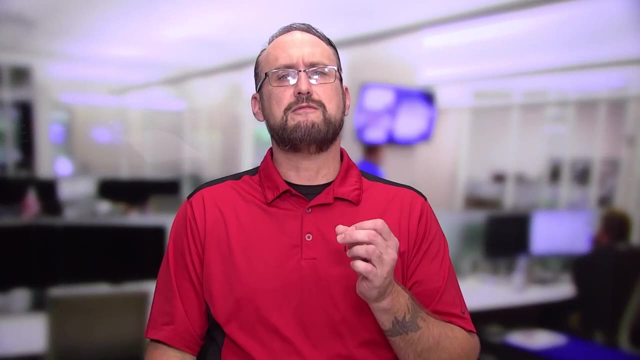 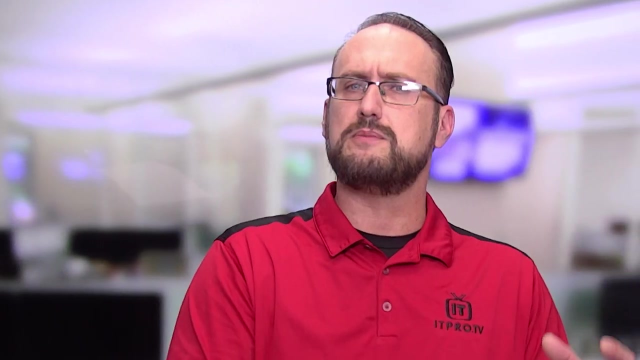 And some of those limitations with traditional software is even being able to analyze the information and make sense out of it. But then, like you heard earlier when we talked about the variety, right, various types of data. See, there's structured data, more traditional data is structured and we can put it in tables with rows and columns in a database and we query against it. 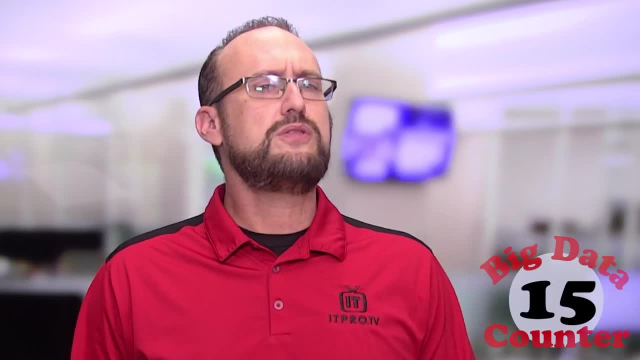 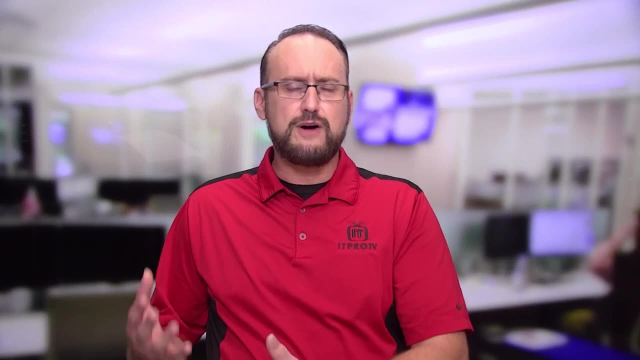 We can use that information, But in big data there's more than just structured data. There's structured information, There's semi-structured information, like JSON, if you will. There's also things like video files that are unstructured, And that presents a challenge. 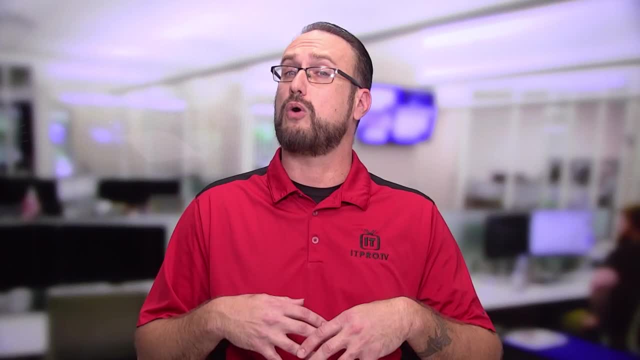 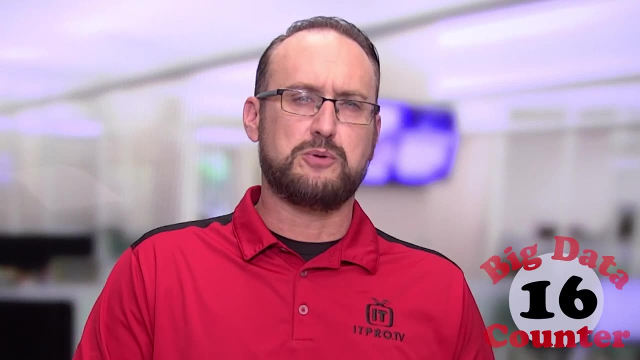 How can we spot the relationships and that statistical analysis across different types of information? So, now that we have an insight into what big data is, let's shift gears a little bit and let's discuss some of the technologies that allow us to work with big data. 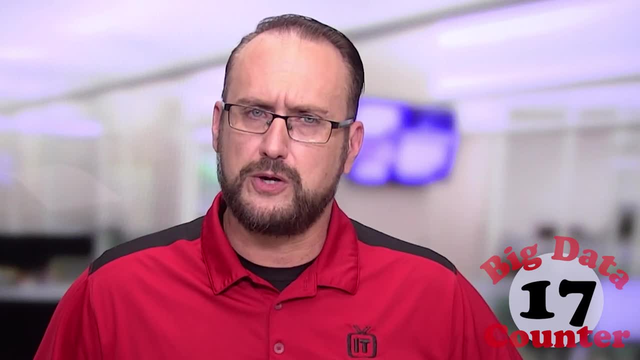 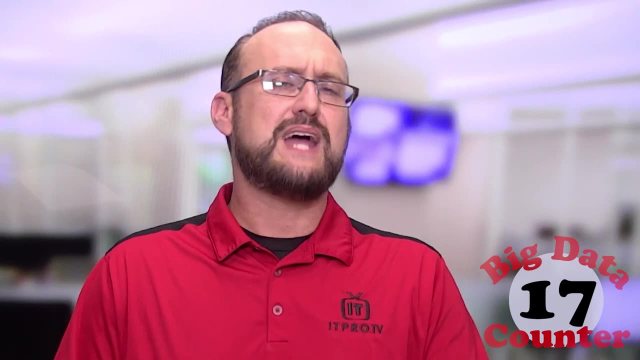 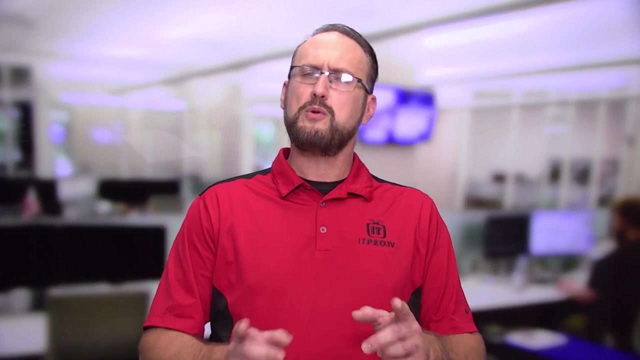 For example, one data specific technology you've probably heard of is Hedis. It's an open source framework and it allows for the processing and storage of big data applications and can handle almost limitless concurrent tasks. Then there's Apache Spark. Remember we talked about IMDB?